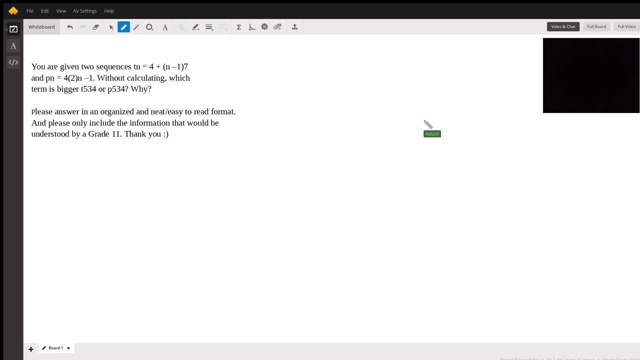 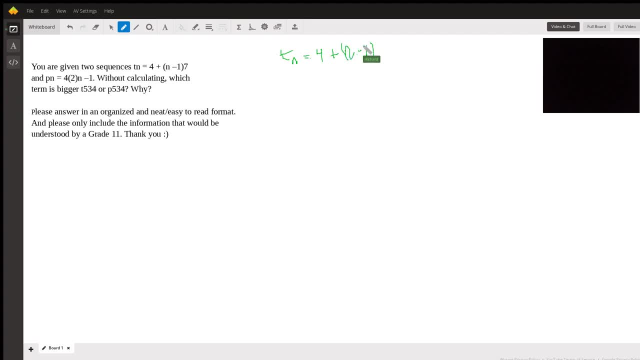 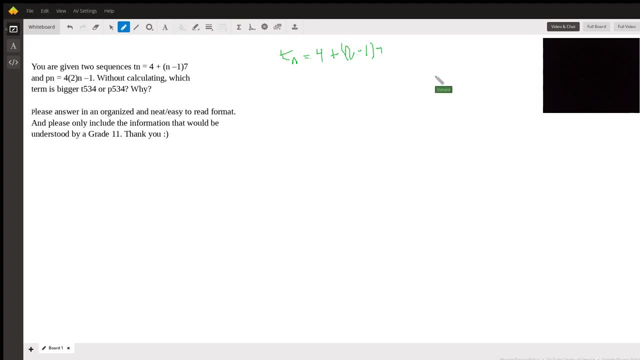 And you can tell it's arithmetic partly because it's linear. And you can tell it's arithmetic partly because it's linear. if we were to graph this and we were to look at: oh, here is T, sub n, here and n, when n is there, is there might be a 0, but we're just start n at 1 here I'm. 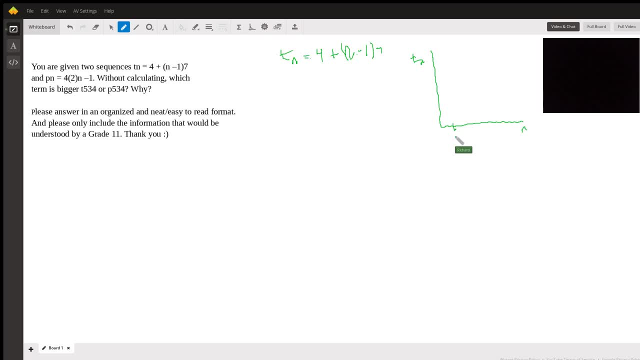 going to start a graph at 1. sometimes they want you to start at 0, sometimes at 1. it doesn't. it doesn't make any difference. 2, 3, so let's just plug this in. so T sub 1 is going to be 4 plus 1 minus 1 times 7. so this is going to be: 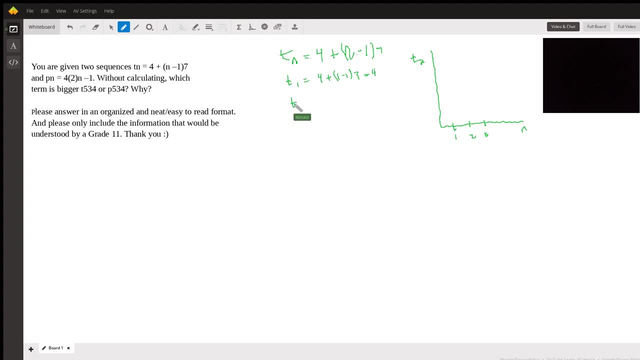 4 and T sub 2. it's going to be 4 plus 2 minus 1 times 7, so it's going to be 11, and T sub 2 is going to be 4 plus 2 minus 1 times 7, so it's going to be 11 and T sub. 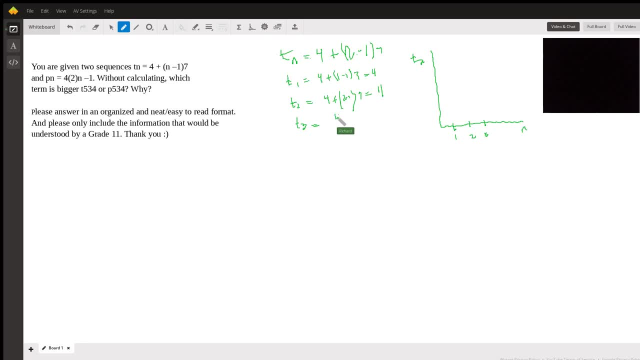 sub 2 is going to be 4 plus 2 minus 1 times 7, so it's going to be 11, and T 3 is 4 plus 14, so it's going to be 18. you can see that every time the value of 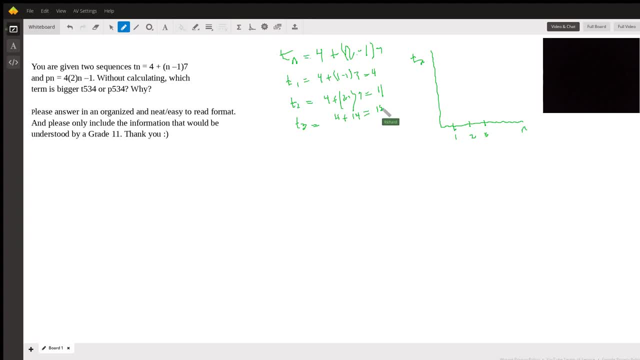 T is going up by 7. you can think of this as a slope of 7, but basically you're just going to have something that looks like this: it's going to be a straight line. it's a linear relationship between N and T. now the second one is geometric. 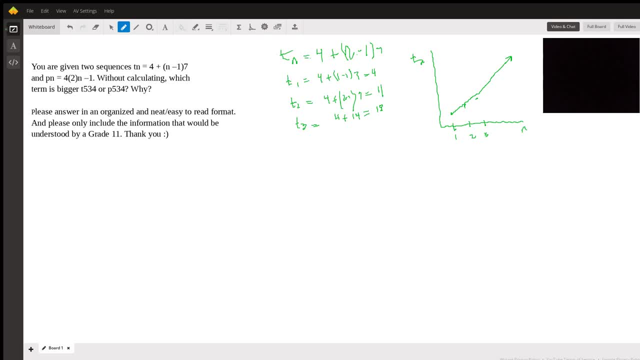 and you can tell because it's not linear, let me change. let me change colors here, because this one unfortunately didn't come out very well. P sub n is 4 times 2 to the n minus 1 power. P sub 1 is 4 times 1, which is 4. P sub 2 is 4. 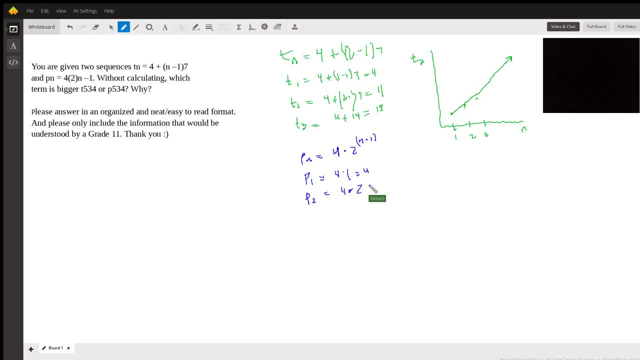 times 2, which is 8. piece of 3 is 4 times 4, which is 16. okay, another way to recognize the geometric sequence is that each increase is multiplied, so it's it's every time. here, you see, it's times 2 times 2 times 2. that's called the common. 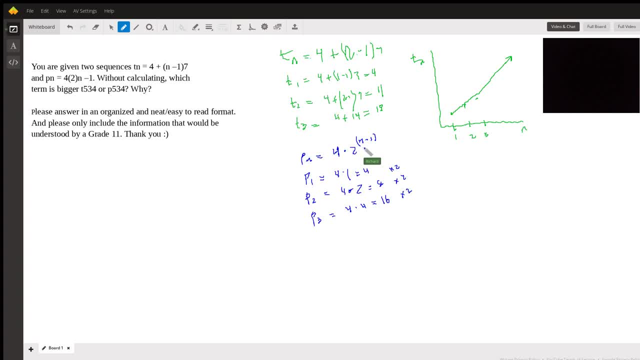 ratio, which is R in in this equation, is 2 up here, you see, the values are changing by the same amount. so, going back to this one, oh, this is plus plus 3. you see, plus 3, that's called the common difference, and so that's the. 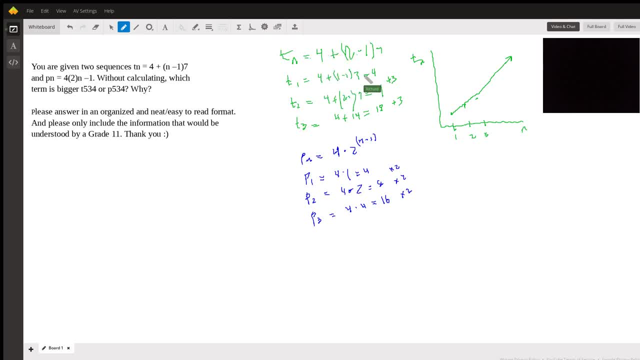 characteristic of an arithmetic sequence is that you have a common difference. a characteristic of the geometric sequence is that you have a common ratio. if we were to plot the blue line, the first one would be 4, so it actually starts at the same point here and then. 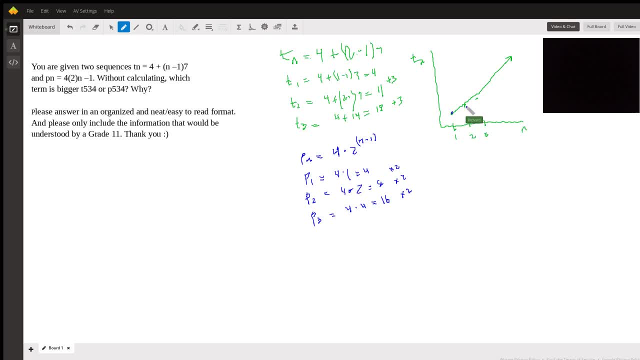 the next next one is 8, the second one was 11, so it's 8 here. it's going to be a little below. and then the next one is 16, which is still a little bit below. but this is going to. this is going to go. if I think we plot another point here, P 4, it's.